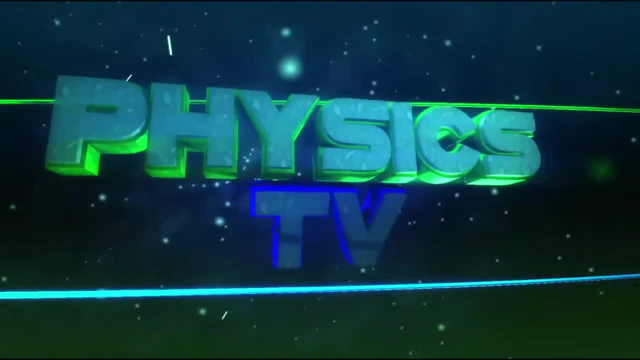 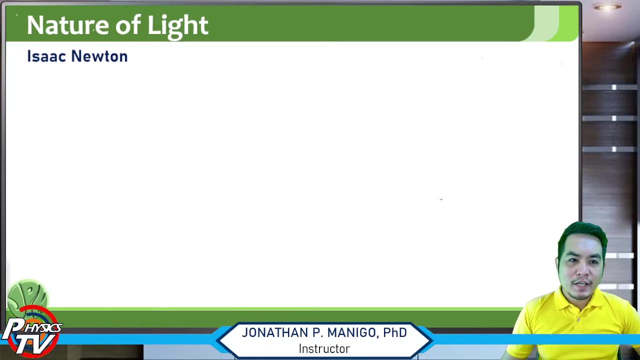 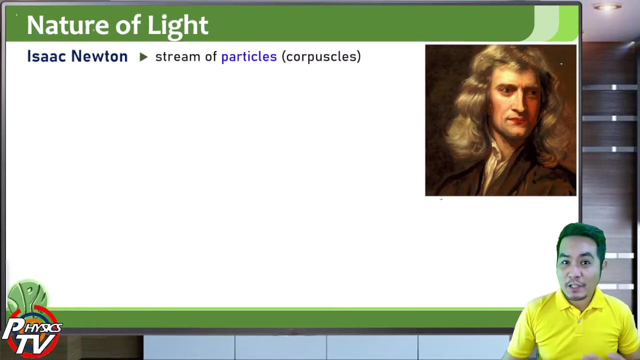 So light? let's first discuss how light. the concept of light was created. So Isaac Newton theorized that light is a stream of particles and he actually termed those particles as corpuscles. Now, in 1670,, in 1665, evidences: 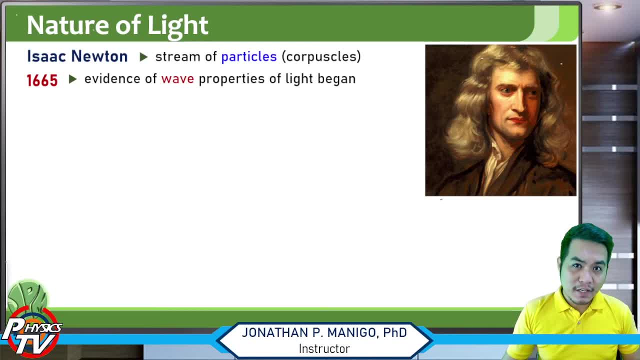 due to experiments done by scientists, evidence of wave properties of light began. So Isaac Newton theorized that it's a particle, But in 1665, evidences emerged that light is also a wave. In 1887, Hertz showed that light is an electromagnetic wave. 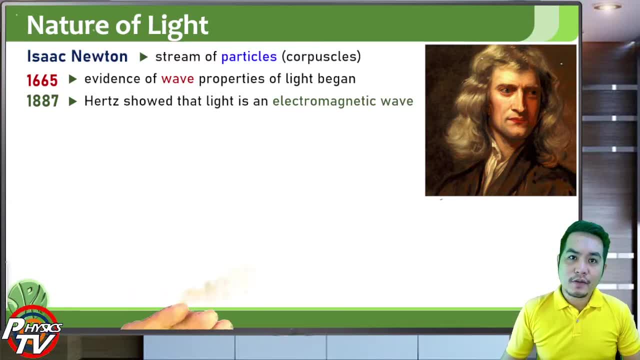 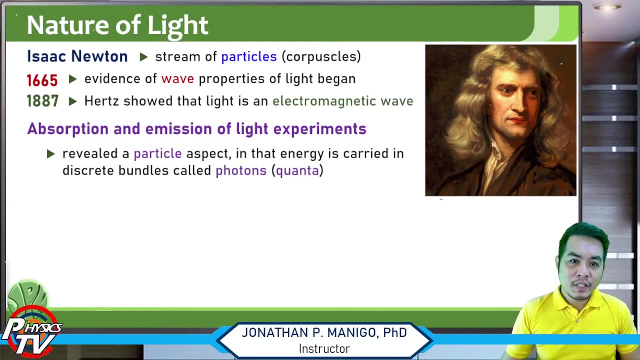 So it now adds further to the, to the, to the nature of light, that it is indeed a wave. Now, absorption and emission of light experiments revealed that light is also a particle. So the energy carried of this particle is in discrete bundles, and this bundle, or this quanta, is what we call photon. 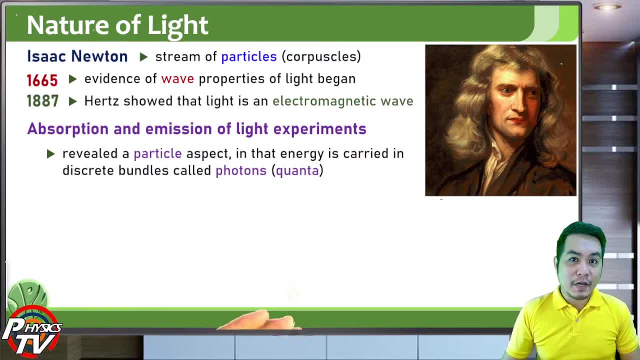 So basically you can describe light as a particle in terms of photons, One bundle of energy And that's basically you can tell that that's one particle of light, a photon. So light is actually a dual, It's both a particle and a wave. 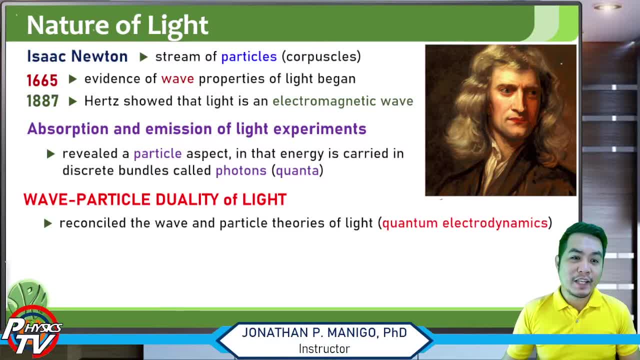 And we call this property, this nature of light as the wave-particle duality of light. So the wave-particle duality of light reconciled the wave and the particle theories of light, And this is discussed specifically in this higher physics subject or high advanced physics subject called quantum electrodynamics. 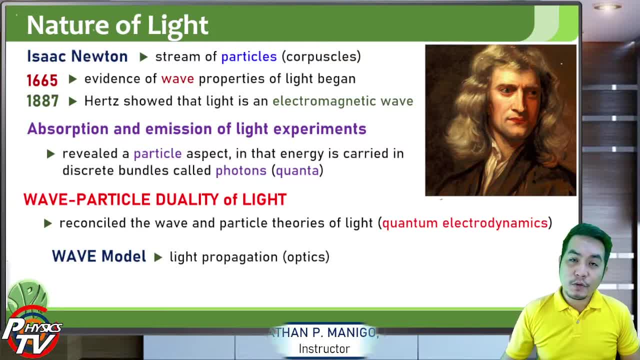 So the wave model of light can be used if you're just studying light propagation or optics, especially geometric optics, And the particle model of light can be used when you are dealing with absorption and emission of light. So you can use both- either of the models, depending on the situation. 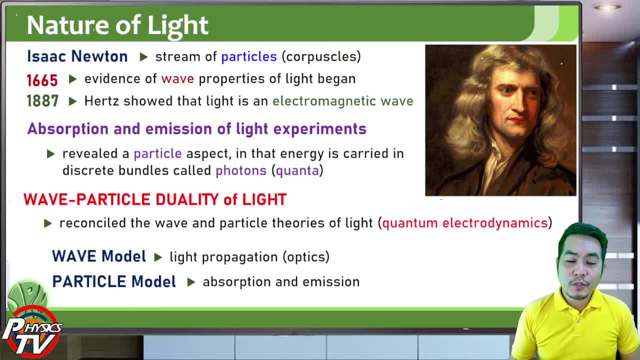 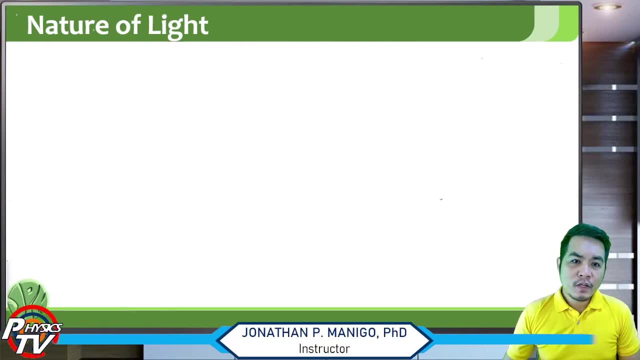 depending on whether you're just studying how light behaves, how light propagates through a material, then you use the wave model. But if you are trying to discuss about the absorption and emission of light, then you use the particle model. So light 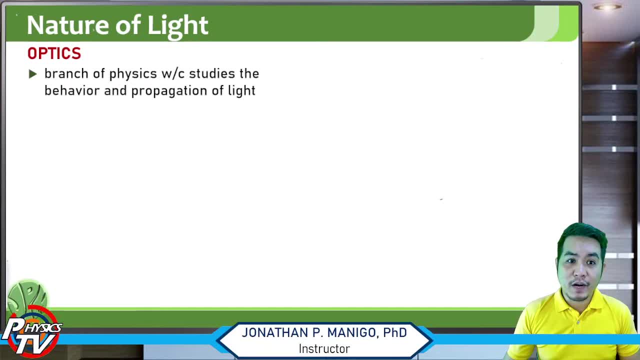 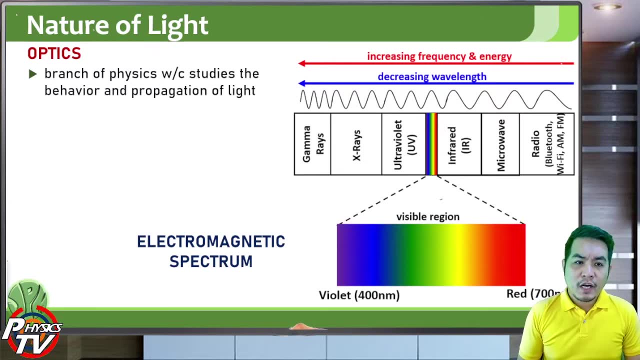 the study of light is basically optics. It's a branch of physics which studies the behavior and the propagation of light. So before we study optics, which is the last chapter of this course, let's first take a look at the spectrum of light. 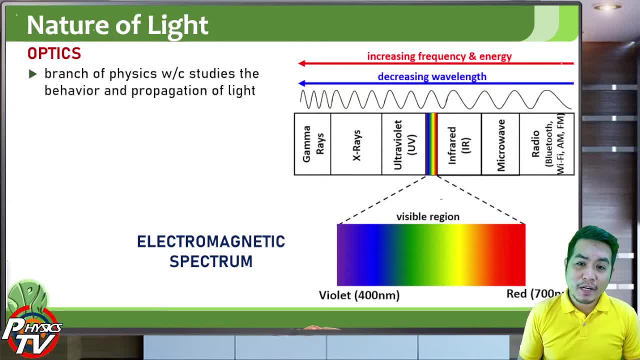 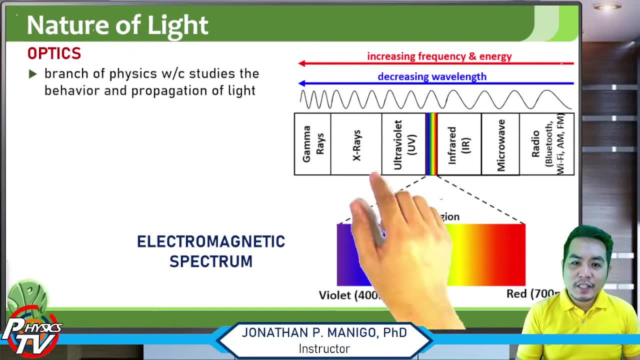 So light is an electromagnetic wave, It's an electromagnetic radiation, And the light that we can see, the white light and the colors, are just a very tiny, very small part of this whole spectrum. So the visible region, the light that we can see, 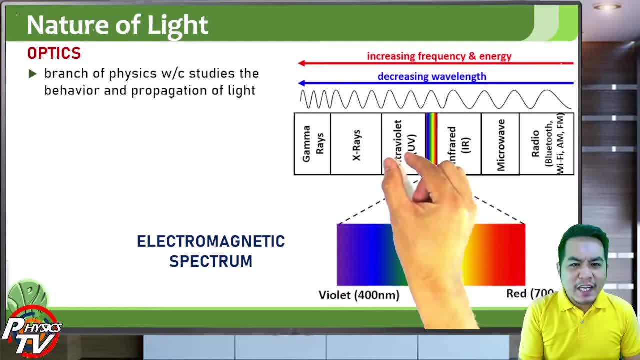 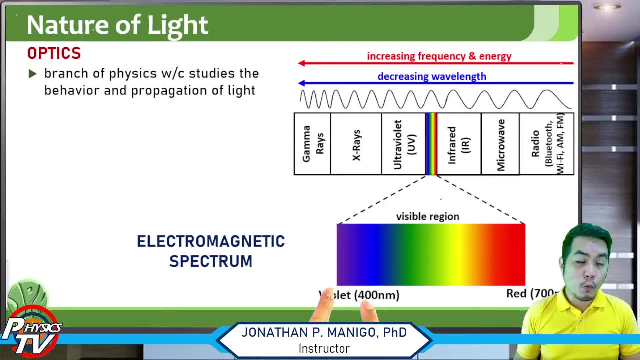 that can be seen by our eyes is just a very tiny part of the whole light spectrum, So what we can see is from violet- that's 400 nanometer wavelength- to 700 nanometer wavelength, which corresponds to red. That's the only region that's visible to our eyes. 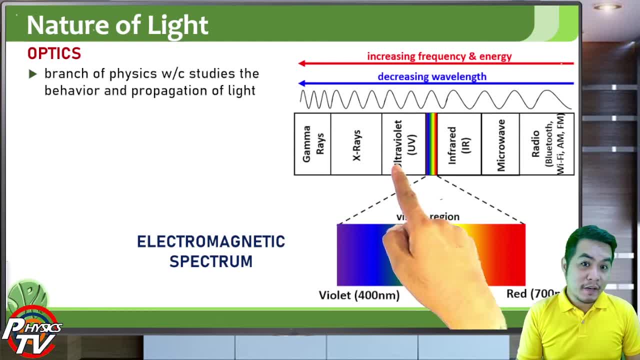 Beyond violet that's now ultraviolet, And beyond ultraviolet you have X-rays, And then beyond X-rays you have gamma rays, So decreasing wavelength it's actually increasing energy or frequency and energy. So ultraviolet light has much higher energy than visible light. 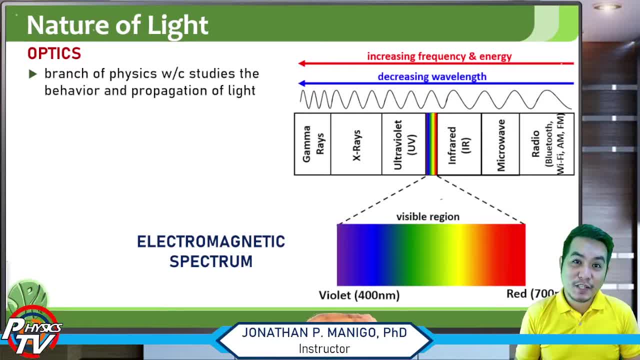 So UV from the sun actually can cause cancer because of the energy and how much more X-rays and how much more gamma rays. So if you're exposed to gamma radiation, you will surely die, Unless, of course, you're the incredible hook. 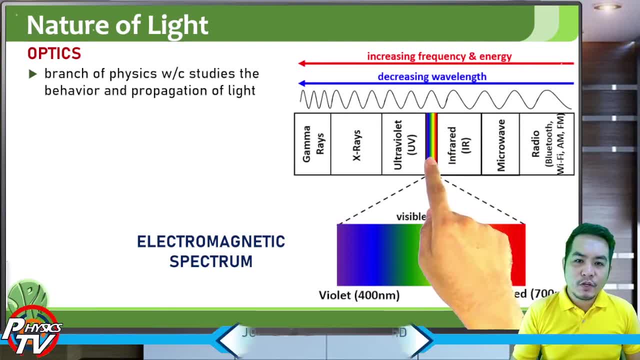 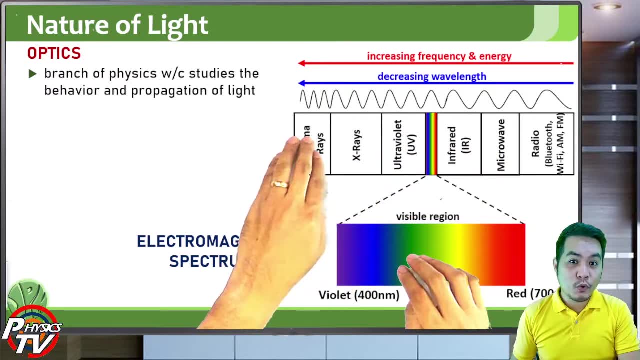 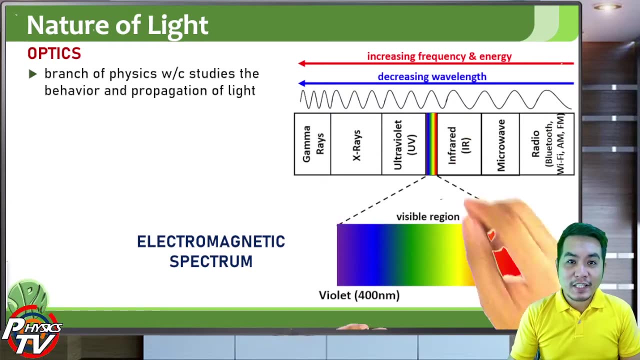 Okay, So beyond red you have infrared Again: UV, X-rays, gamma rays. these are now outside the visible region of light. You can no longer see this light, Similar with above, the red light. So infrared, we cannot see infrared. 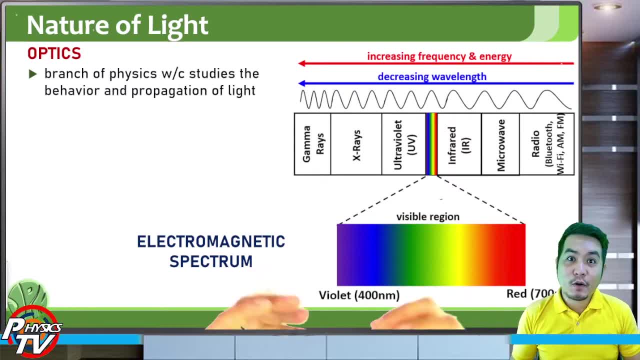 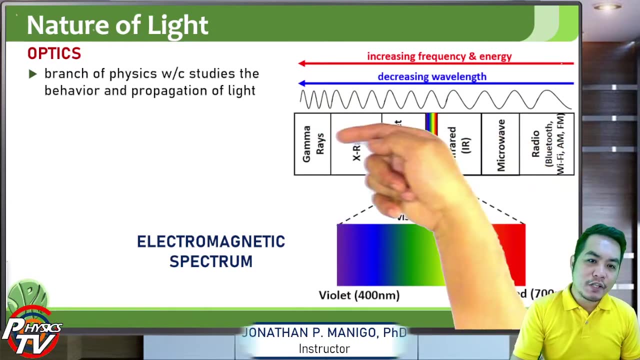 but we can feel it as heat. So infrared is also in our remote controls that uses infrared Microwave. it's much higher than sorry, much lower energy. So increasing energy towards gamma rays. This is actually decreasing energy in the opposite direction. 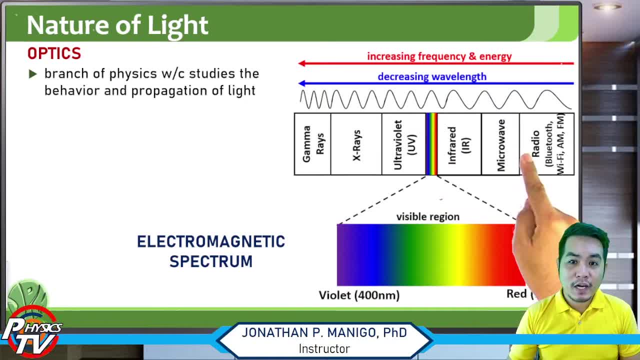 So basically infrared, microwave and radio waves, radio waves that includes Bluetooth, Wi-Fi, AM, FM. those are radio waves And they're actually very low energy, low frequency and low energy- electromagnetic waves or light, And we cannot see this light. 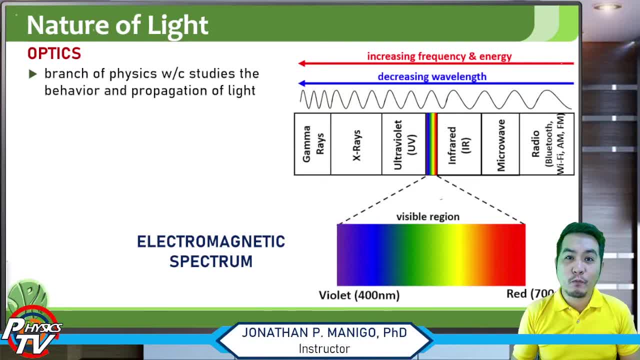 We cannot see an AM radio wave, an FM radio wave, We cannot see Bluetooth, We cannot see Wi-Fi, Because those are now beyond our visible capacity, of our eyes. Now, even though these are lower energy wavelength, there's a certain region here. 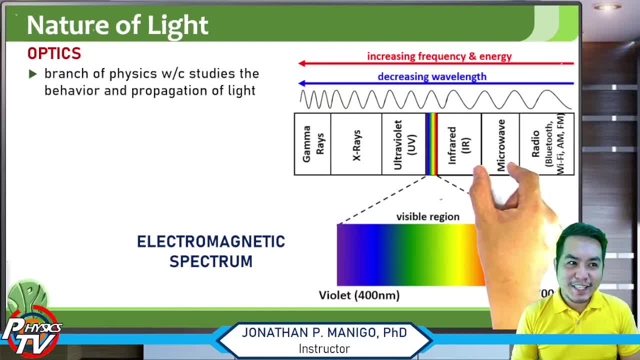 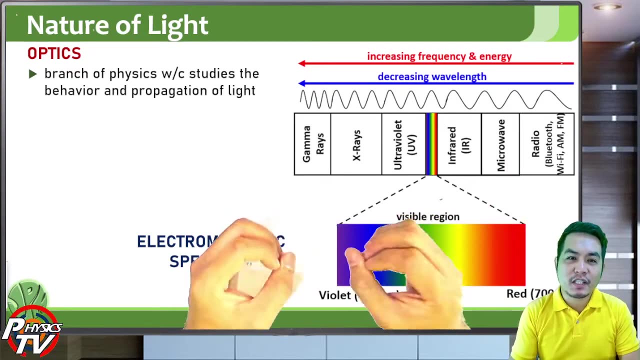 the microwave region, which is harmful to us Because microwave, or rather water, is very sensitive to microwave. When you microwave water, water will start to boil, Water will start to water, molecules will start to get energetic. Water actually absorbs microwave. 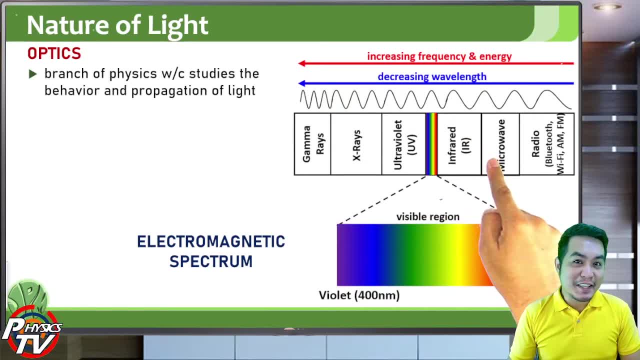 So microwave is lethal or it's harmful to anything that contains water. So if you just want to heat your food in the oven, you can use microwave oven to heat it. But if you, if you place a, a being, a live. 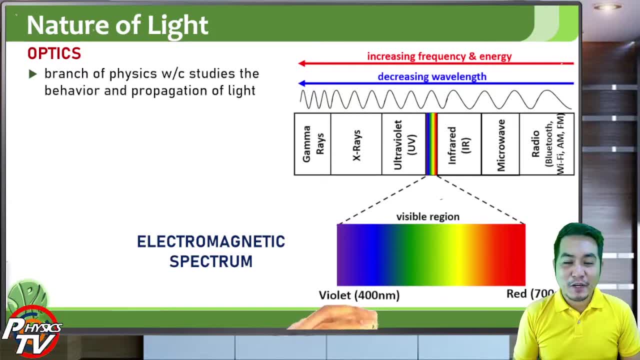 a live being there or a human being, you will surely die Because our bodies are made of 75% water. So there's just a specific frequency for microwave that our bodies or water will react to. So microwave is harmful to anything that contains. 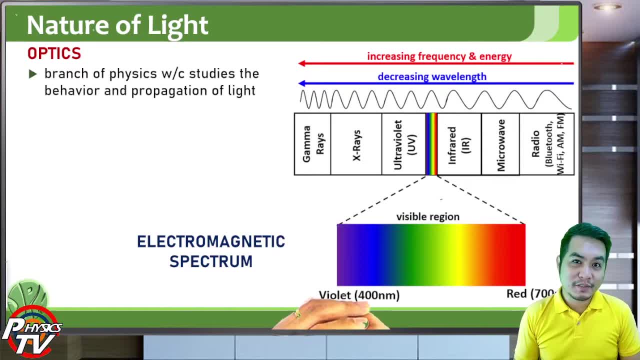 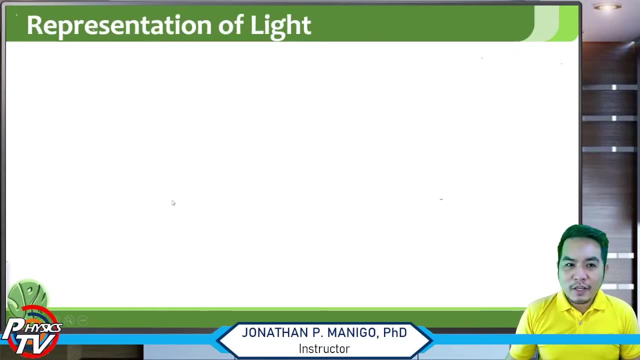 or it makes water boil. Microwave makes water boil, So since we are made of water, our water in our body will boil. We will die, We are exposed to a higher dose of microwave. Okay, So there are many ways to represent light. 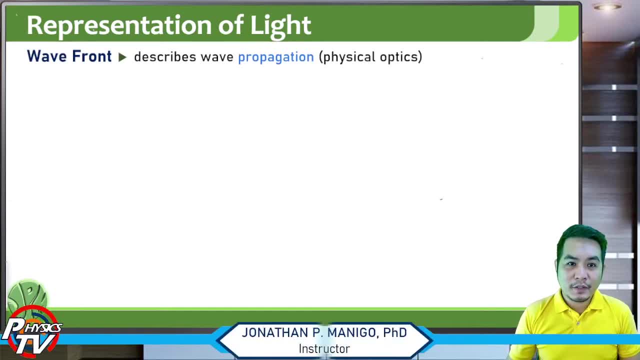 We can represent light as a wave front, So this a wave front describes the wave propagation of light, So physical optics. it can represent the wave's crest or the wave drops, So similar to sound, sound is a wave, Light is also a wave. 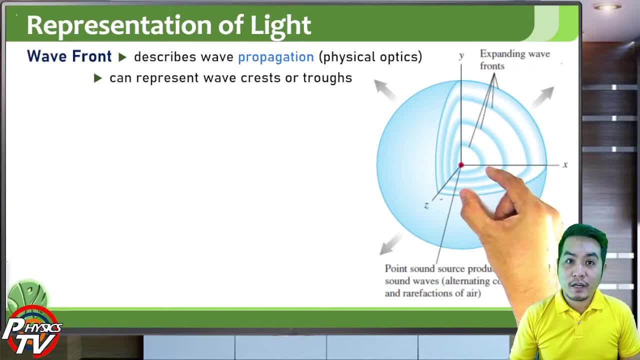 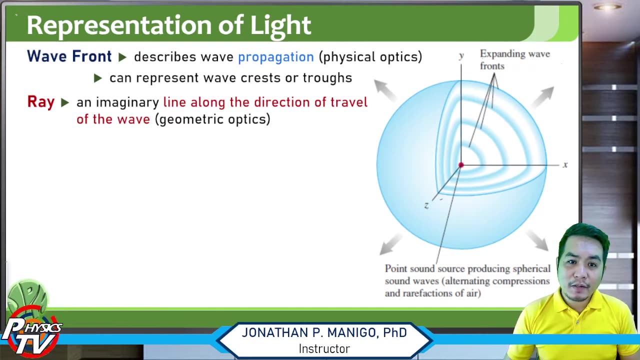 So the wave fronts are the- yeah, the crest and drops of the waves are actually spherical, or the wave fronts are actually spherical in nature. So we can also represent light as a ray, So an imaginary line along the direction of travel of the waves. 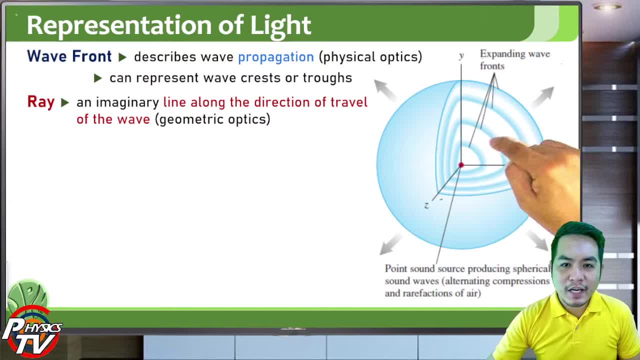 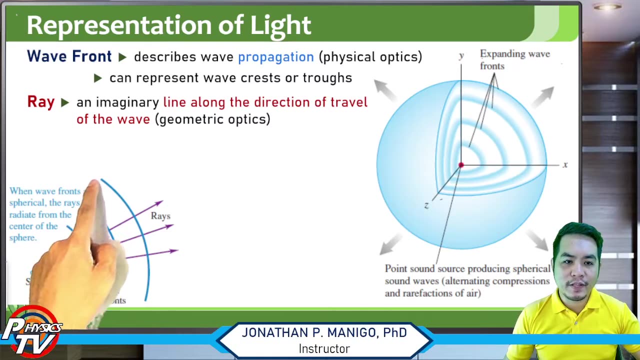 So in this case this is the ray, An imaginary line along the direction of the travel of the wave. So that's basically geometric optics. So the relationship between wave fronts and rays is, if this curves, here the spherical curves, here are the wave fronts. 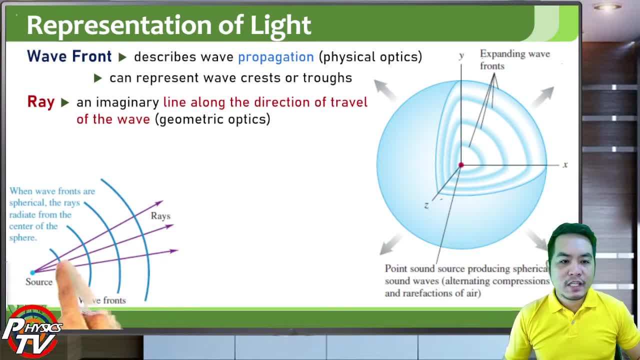 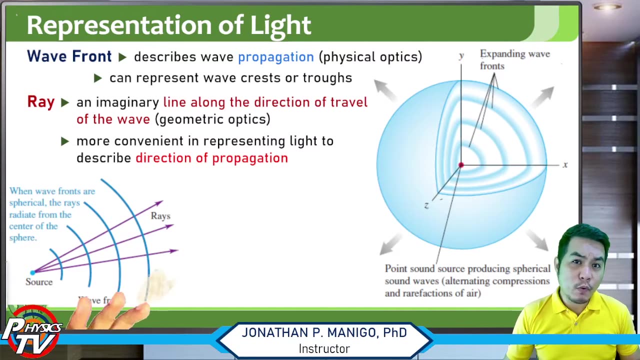 then these lines here, which is always perpendicular to the wave fronts, are the rays. So the rays are always perpendicular to the wave fronts And instead of representing light as wave fronts, it's actually convenient- more convenient- to represent light in terms of rays. 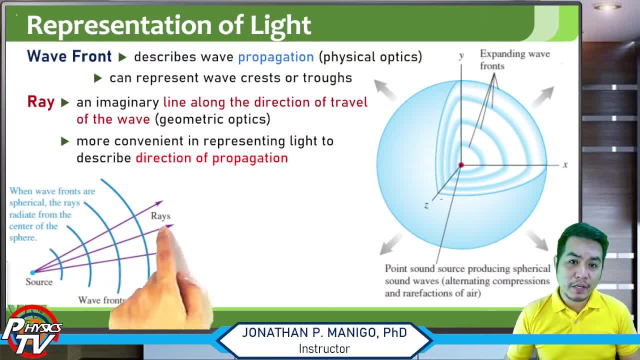 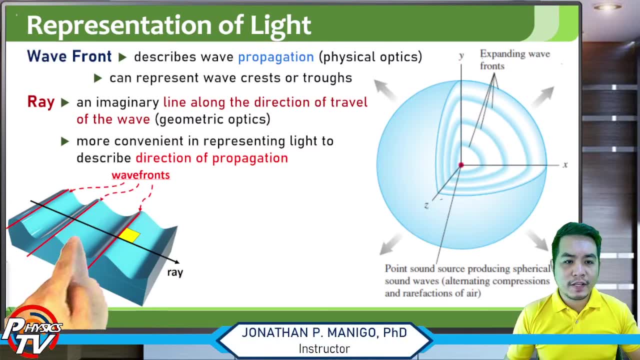 Because you're just looking at the direction of the propagation. So, if you have, if this is your sorry electromagnetic wave, these are your wave fronts and the ray will be perpendicular to that wave front. So always, wave fronts and rays are perpendicular to each other. 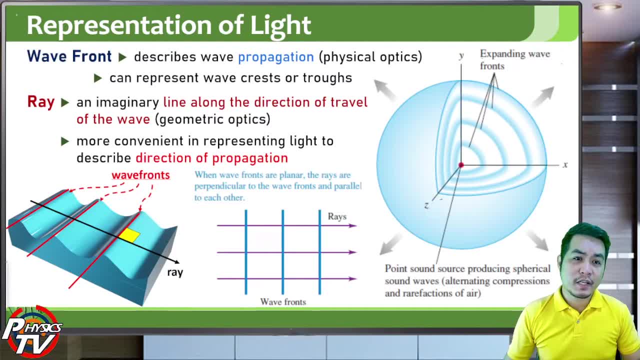 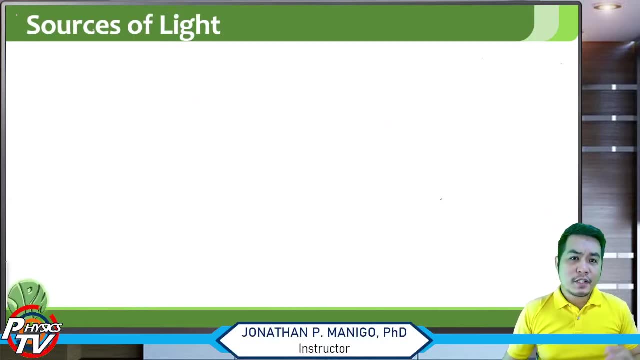 So, from this moment on, we'll just represent light using rays. But that means that if we have a ray in this direction, that means that there will be a wave front perpendicular to that ray. Okay, so let's now discuss the different sources of light. 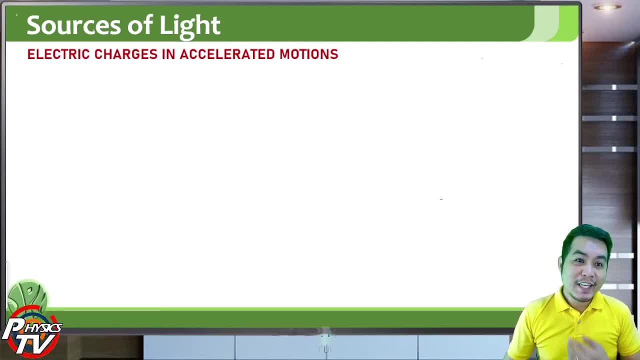 So the basic source of light is electric charges in accelerated motions, Or basically electric charges that are accelerating. When you say accelerating it's either speeding up or slowing down. It must not be moving at constant velocity. So one example of that is an oscillating or accelerating motion. 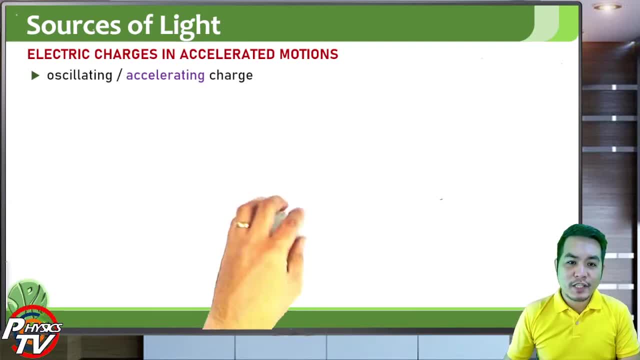 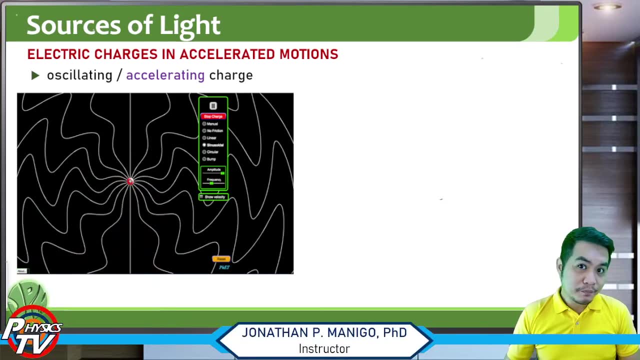 In general. So if you have a charge that is oscillating, say oscillating up and down, take note that a charge has an electromagnetic field. Now if it moves up and down, what will happen to its electromagnetic field lines? It will also wave. 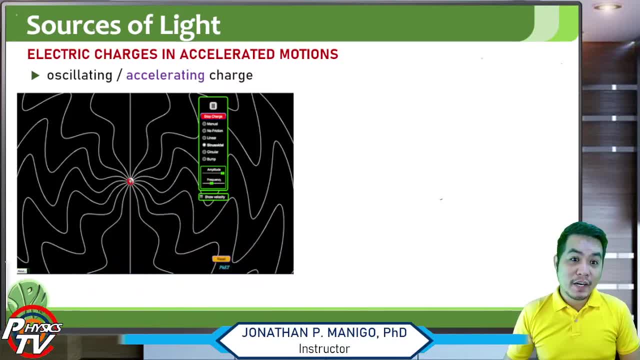 And that basically creates an electromagnetic wave or light. So it's basically just the electric and magnetic field lines that are waving. So if the electric field and the magnetic field lines are moving, the magnetic field and the magnetic field lines are waving to generate an electromagnetic wave or light. 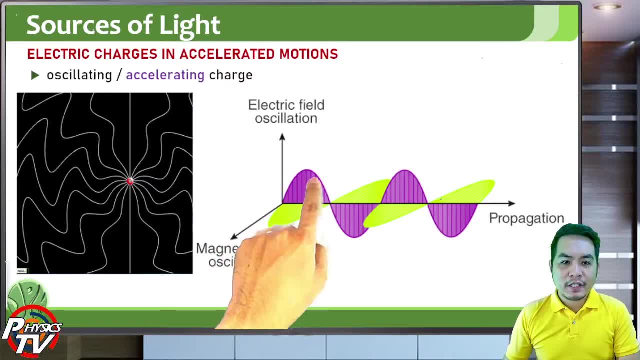 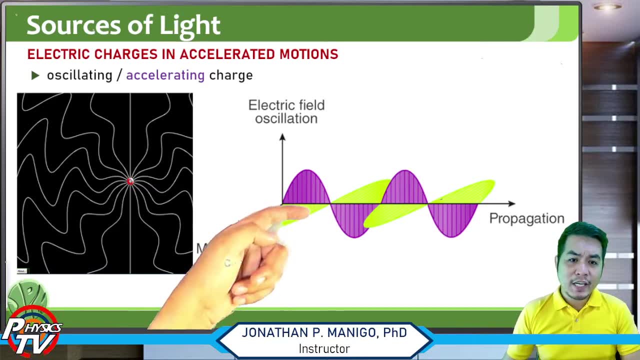 So, basically, the electric field, this is the electric field, the purple one, and this is the magnetic field, the green one. So they are waving, basically, and they are moving. They're waving in this direction And the wave is traveling in this direction. 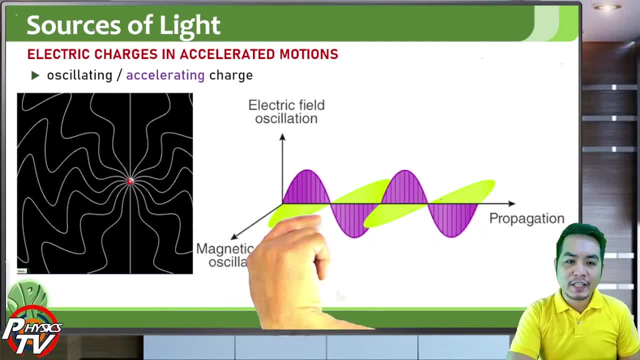 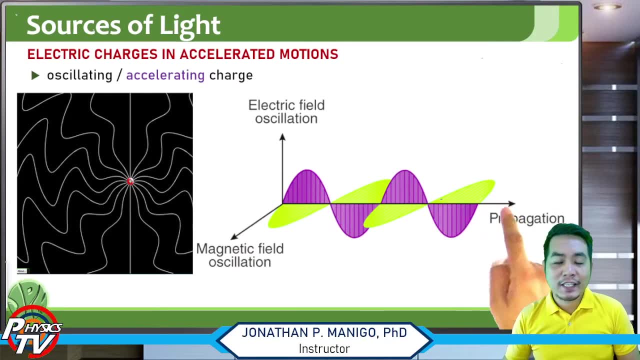 So basically, this picture here will generate light that is moving And this direction is the direction of the ray. So this, you can think of this line as the ray, the direction of propagation of light. So that's the basic source of light. 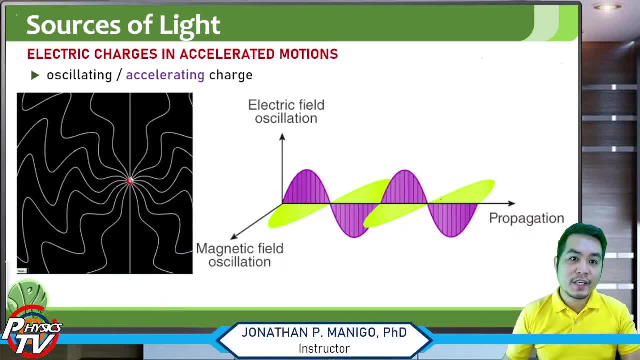 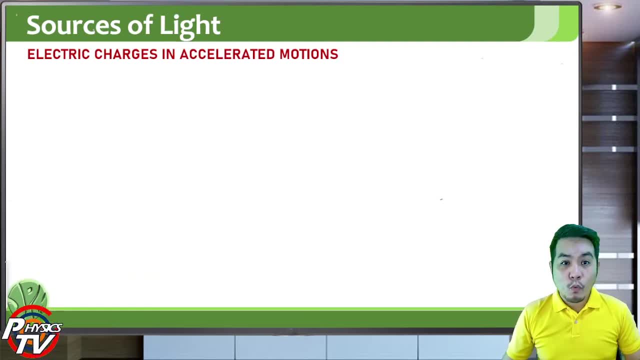 a charge that is oscillating or accelerating, speeding up or slowing down, causing the electromagnetic field lines to wave. So, in general, all bodies actually emit electromagnetic radiation because we are composed of atoms And inside of us we have the electromagnetic field lines. 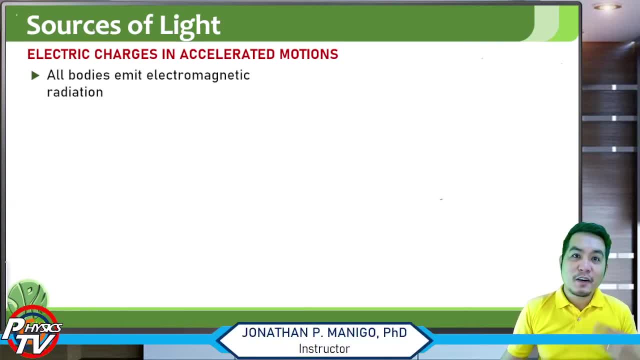 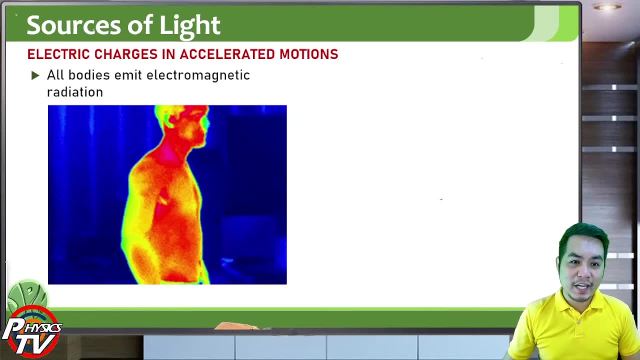 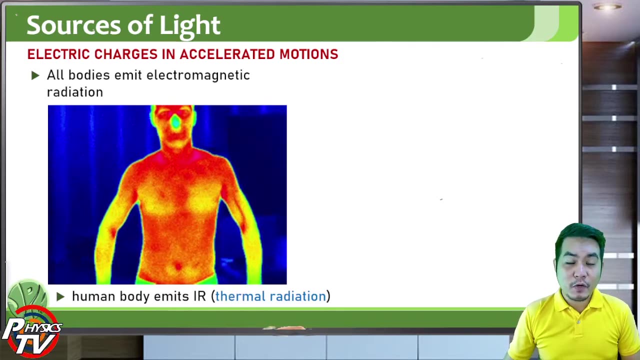 And inside atoms are electrons, And electrons are always moving, accelerating inside an atom. So basically we are generating light. All bodies emit light. So in our case we are actually emitting infrared And we can see infrared if you have a thermal scanner. 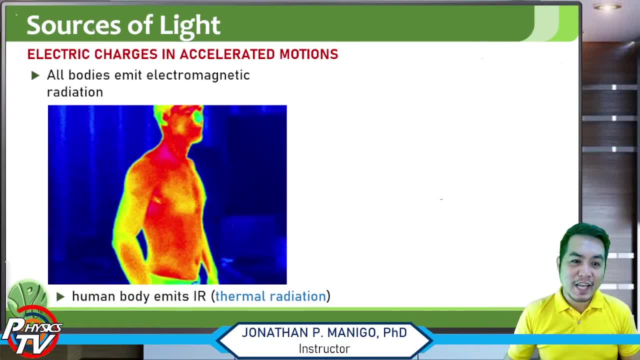 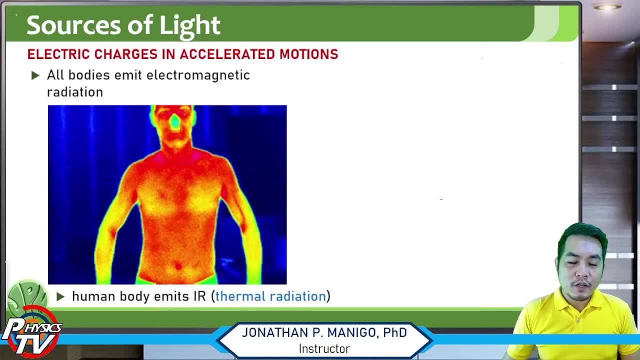 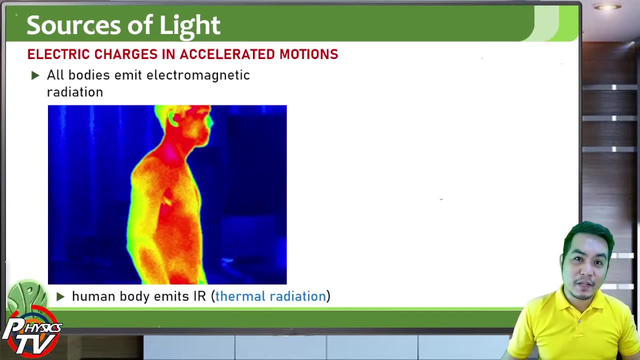 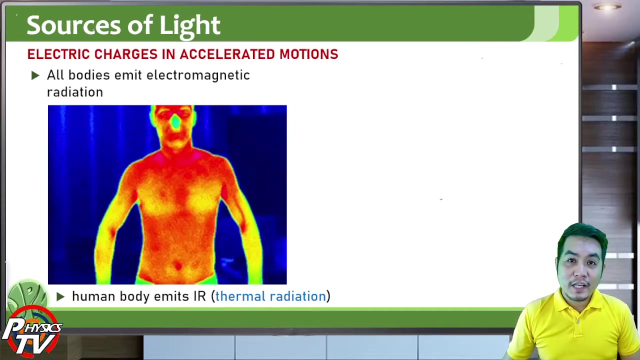 Just like in airport, there are thermal scanners to scan your body temperature. So sometimes you discontinue to emit light only when you're dead. Actually, if you're dead you still emit some form of infrared light, But all bodies emit infrared radiation or infrared light. 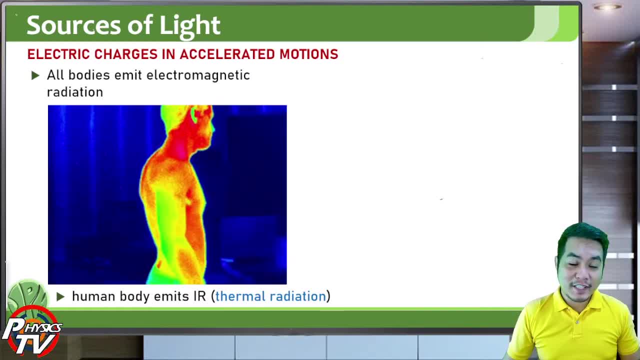 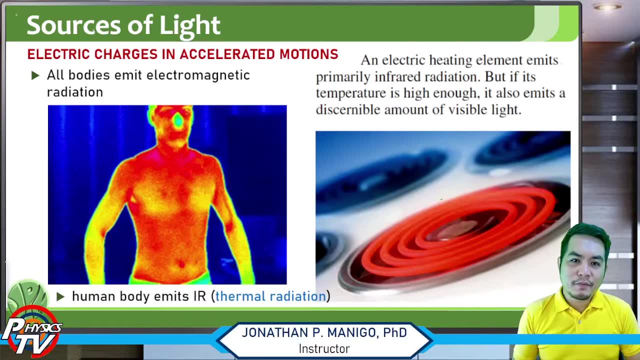 But again it's invisible to us. You need a specific device, such as a thermal scanner, to view that. So this is an example of basically, when you hit something, it actually emits infrared. So, for example, the gas stove. 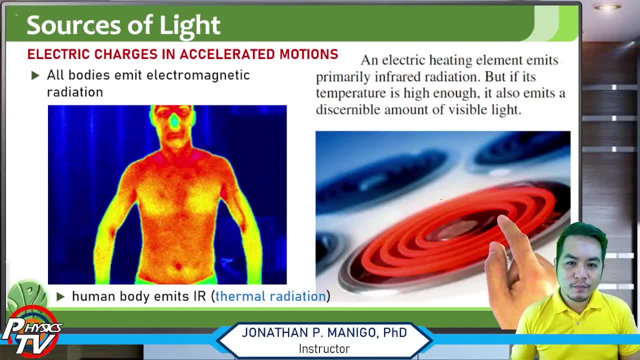 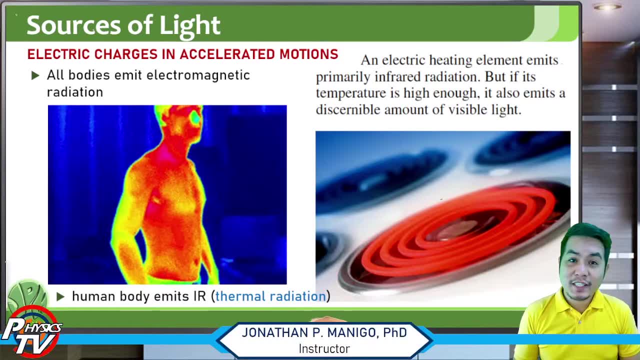 If you hit your gas stove, that will actually emit infrared, But you cannot see it, but you can feel it as heat. So, such as the sun, the sun emits infrared radiation, But we cannot see it. We can feel it, though, as heat. 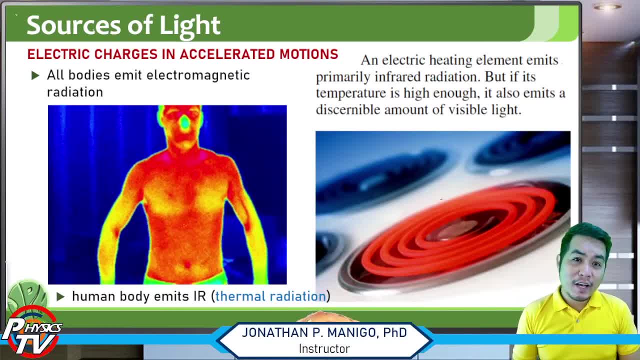 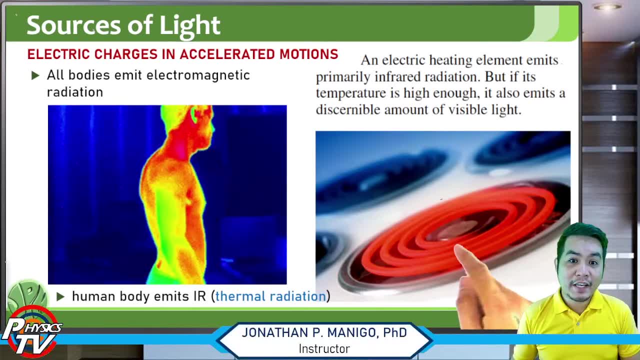 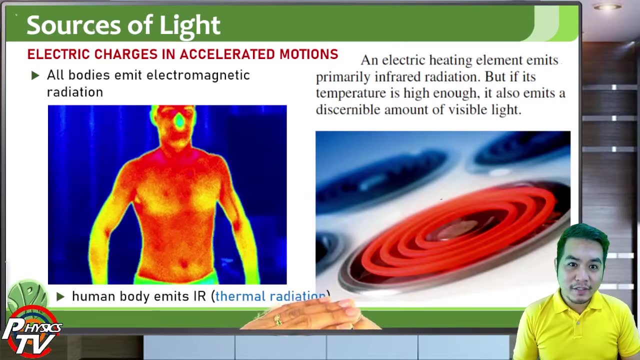 So heat is basically an indicator of thermal radiation. Now, in certain instances, if the temperature of your stove is high enough, it will emit visible light And it will start with red, Red, then orange, yellow, green, blue, violet. 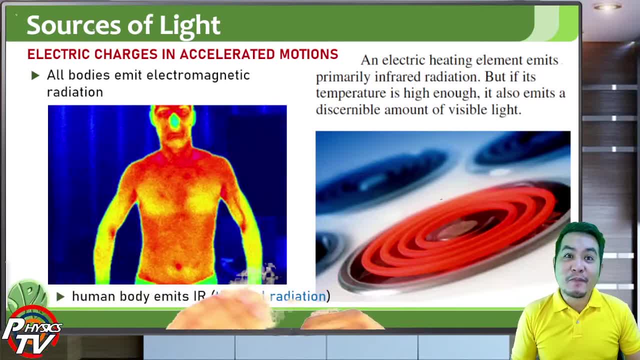 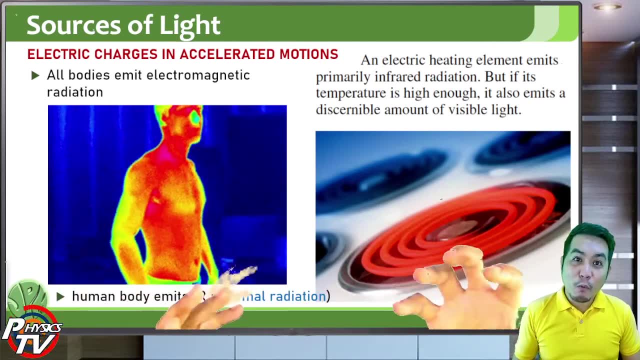 If the color is violet, then that's already very hot, And if the color is white, meaning all of the colors. white is just a combination of all colors. If you see a white light, a white hot object, that's the hottest of all the visible colors. 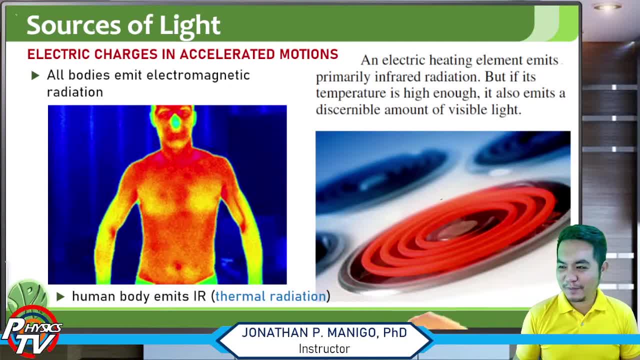 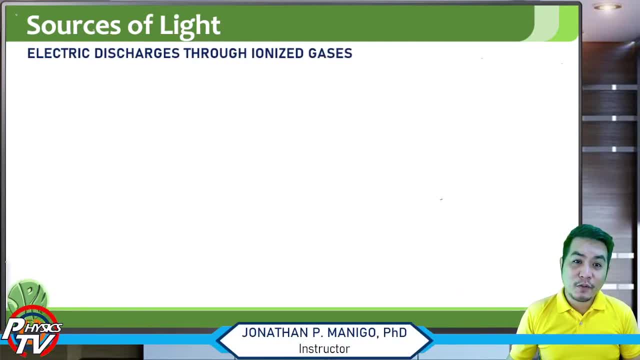 So don't touch a white hot plate, Okay. So other sources of light include electric discharges through ionized gases, So basically this is ionized gases, plasma. So example of this are mercury lamps, fluorescent lamps, stars such as our sun. 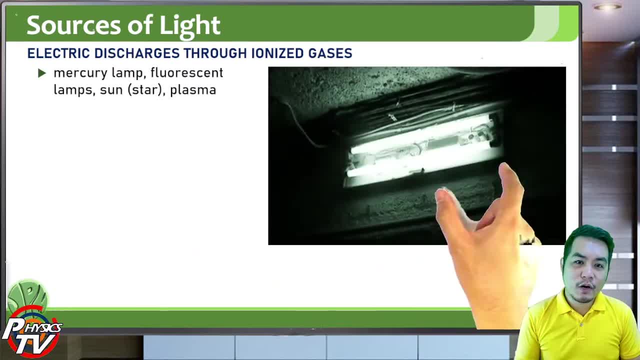 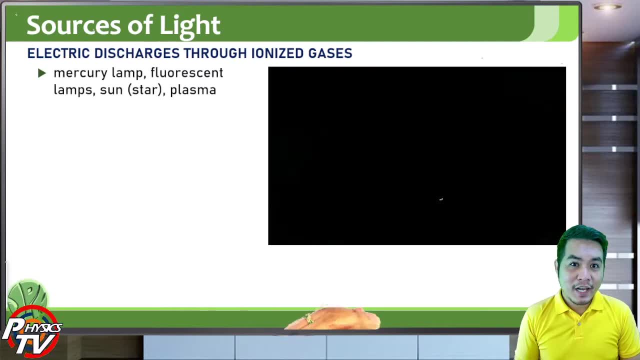 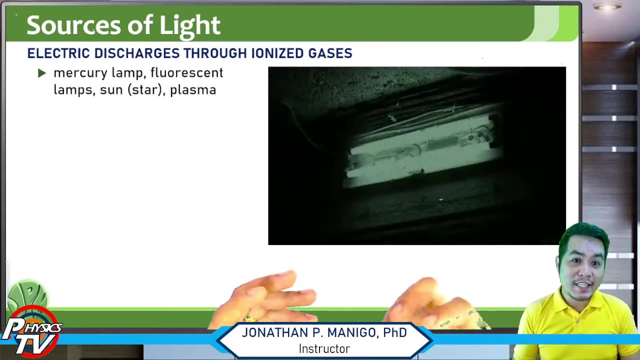 or in general plasma. So usually in our old fluorescent lamps you use some kind of gas there inside And then when you, when electricity flows through that gas, it ionizes that gas, And when a gas is ionized it will discharge. 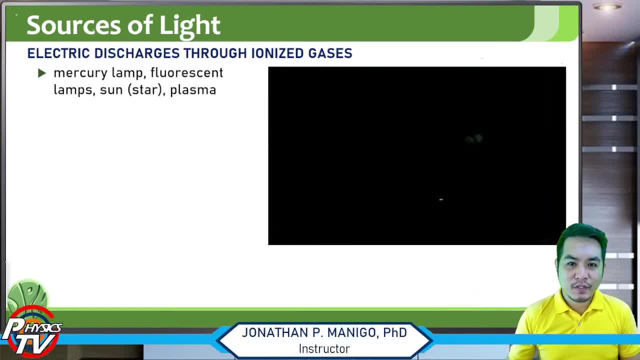 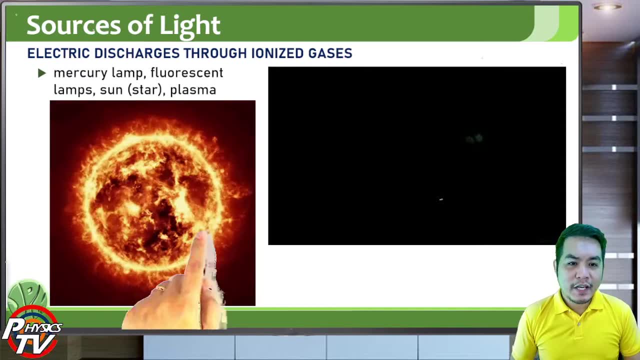 It will emit light. So that's one source of light. So of course, our sun or any star in particular or in general, So they emit. they actually emit the whole spectrum. Some of it are just filtered by our atmosphere, But UV can still pass through our atmosphere. 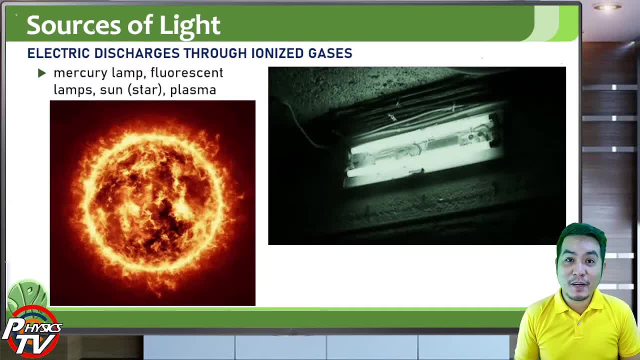 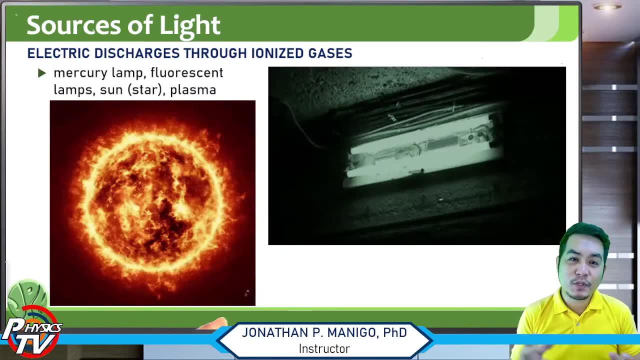 Infrared can still pass through our atmosphere. Visible light can still pass through our atmosphere, So when we look at our sun, it will look yellowish. That's the visible, because the yellow is the most highest intensity that we can see, But it still emits. 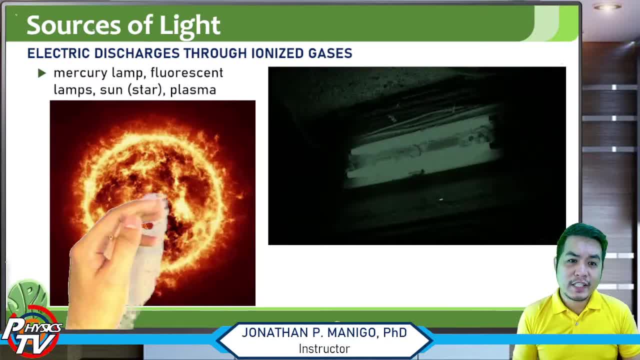 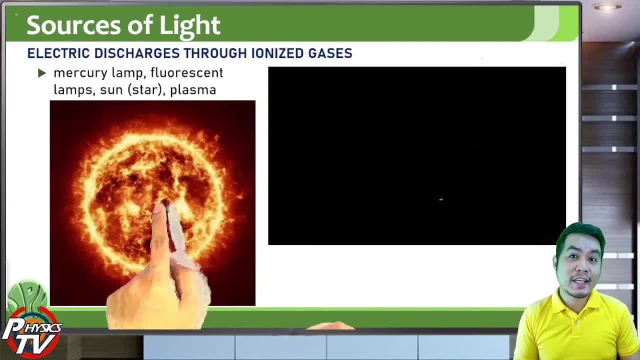 it still emits all of the colors And in fact, it still emits infrared, because we feel the heat of the sun And that is infrared. And it also emits UV, But we don't feel UV. We just know that we have. 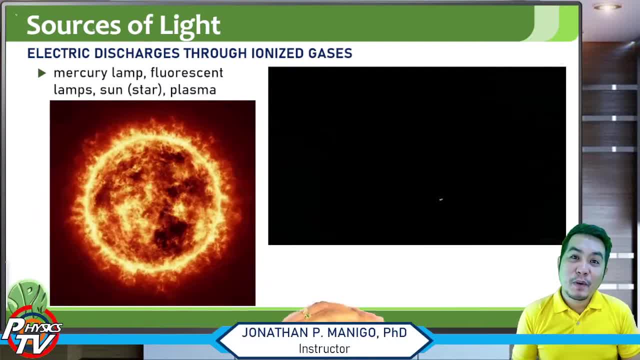 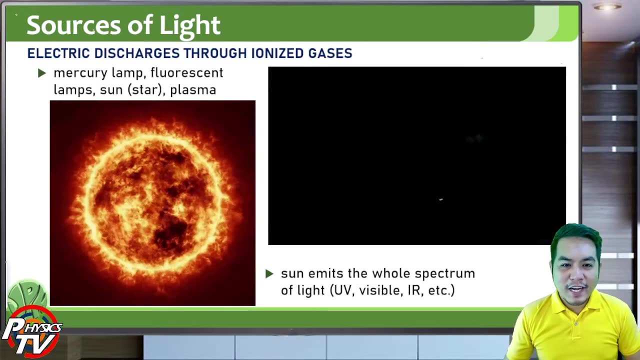 we are exposed to UV when your skin darkens, which leads to basically cancer. So skin cancer are caused by UV exposure from the sun. So the sun emits the whole spectrum of light: the UV, the visible, the infrared and et cetera. 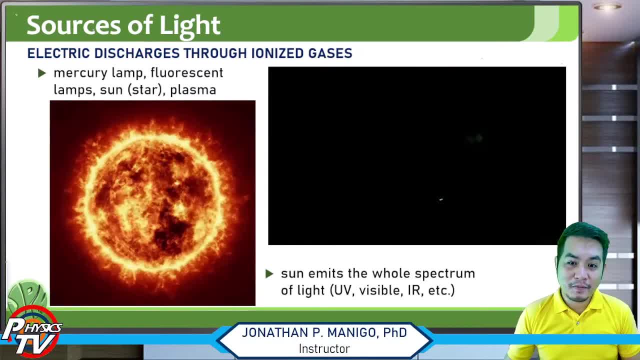 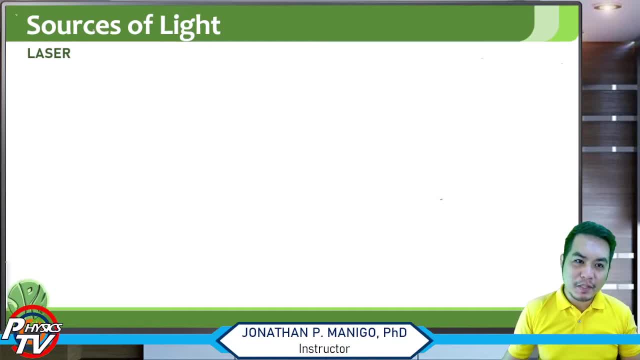 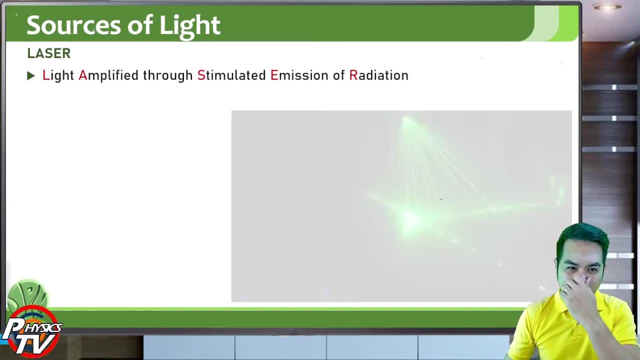 and the other colors, the other spectrum of light. So the last source of light that we will discuss is a laser. It's basically an acronym for light amplified through stimulated emission of radiation. So there are many applications of lasers. So in a laser, 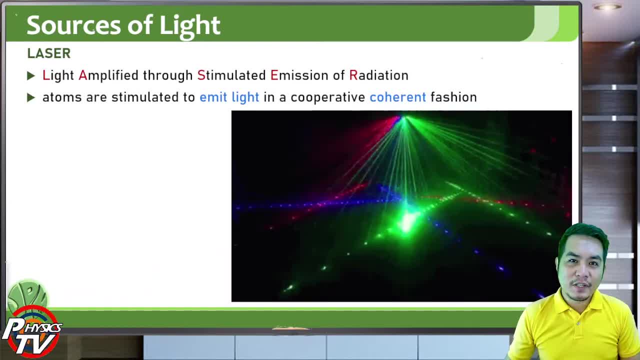 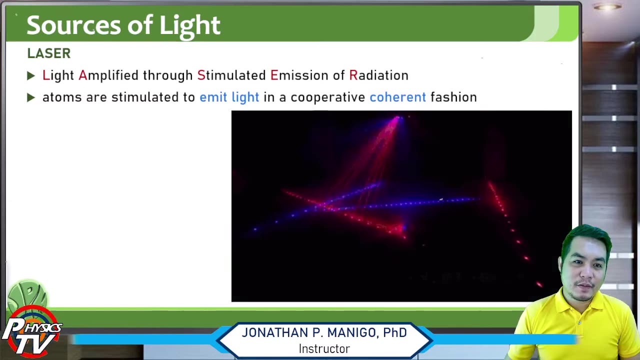 the atoms of the material, whether you use a solid state laser, liquid state laser or a gas laser. so you can have three types of laser: solid state, liquid state or gas. So the atoms in these states or in these spaces. 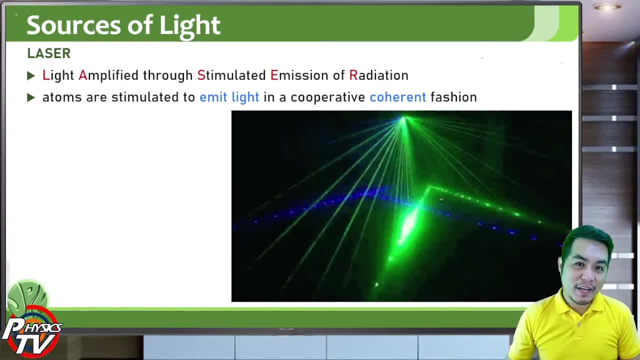 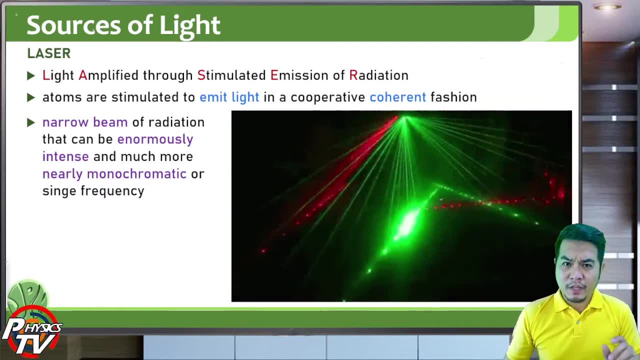 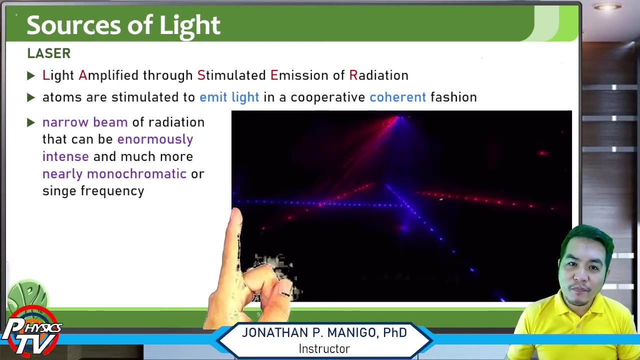 are stimulated to emit light in a cooperative, coherent fashion, And it can produce a narrow beam of radiation that can be very intense And nearly monochromatic- just one single frequency or one color. So that's the advantage of lasers. So lasers has a lot of applications. 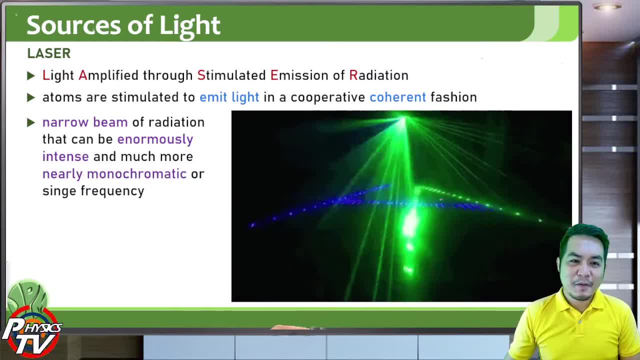 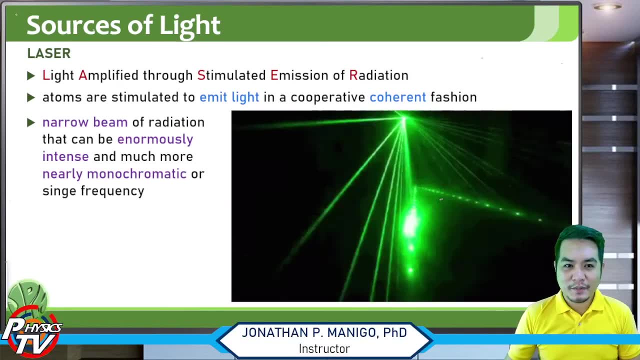 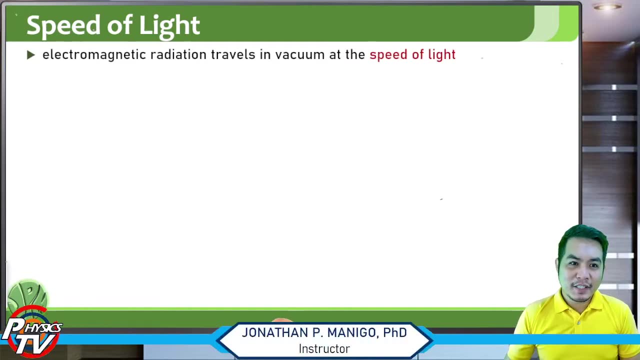 such as these color lights. So there are medical, educational, academic applications of lasers. Okay, Another property of light is the speed. It's speed. So all electromagnetic radiation, or all light that travels in vacuum or in space, in empty space. 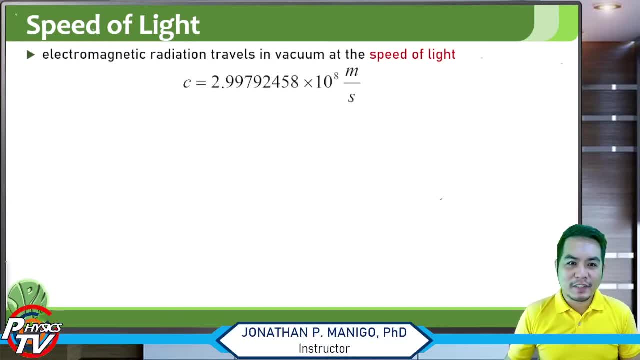 travel at this speed of light, 2.99, or we'll just round off this to 3.. 3 times 10, to the 8 meters per second. So this is what we call the speed of light in vacuum. So this is a simulation. 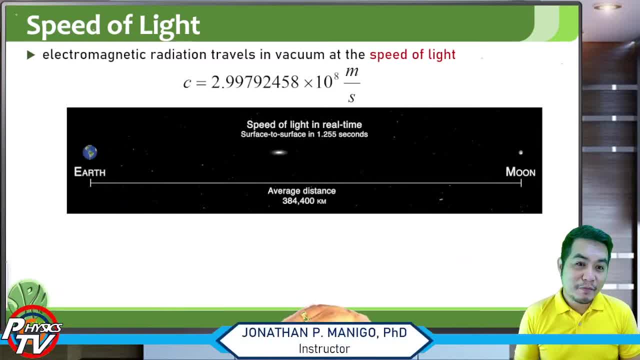 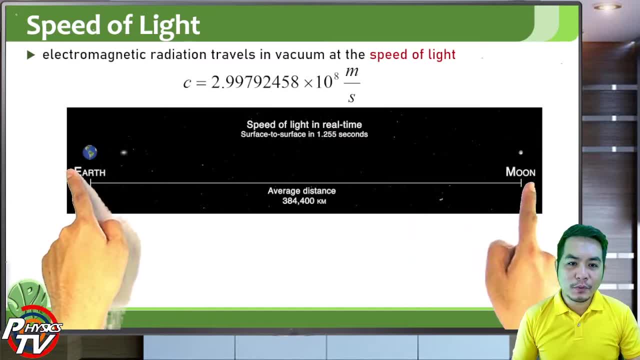 of how fast light from travel is: 3 times 10 to the 8 meters per second. So light actually travels from earth to the moon in just 1.255 seconds. So, as we're talking right now, light is traveling from earth to the moon. 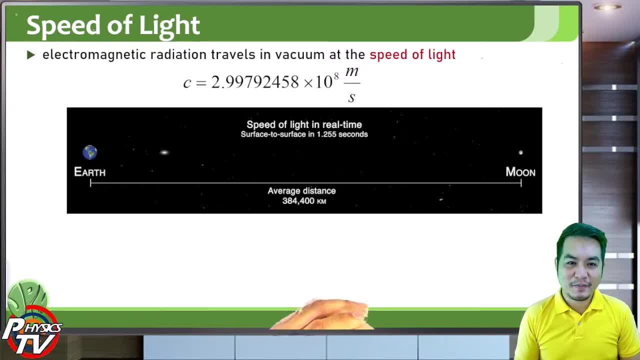 in just 1.255 seconds. So that's actually very fast. This speed is actually very, very fast. So a light from the sun travels to earth in 8 minutes. So that tells you how far the sun really is with respect to earth. 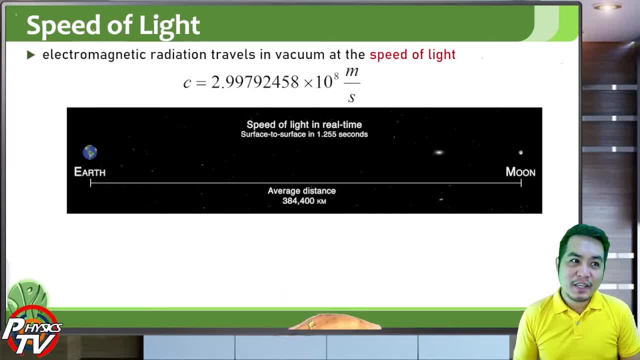 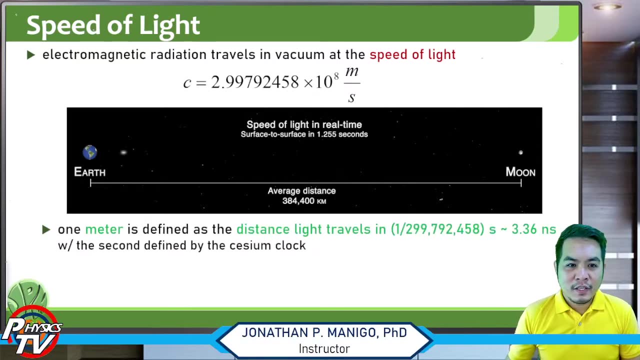 So in the instance that our sun, say say, instantly disappeared, we will still notice that 8 minutes later, because light travels 8 minutes from the sun to the earth. So, based on this speed of light- this is a universal constant- We define 1 meter- 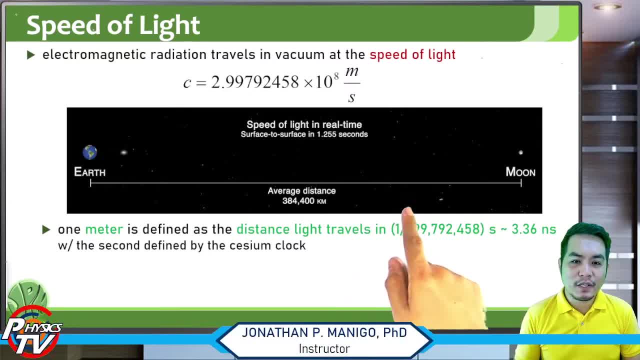 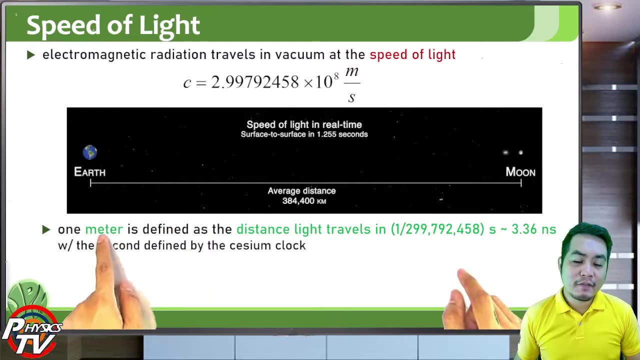 as the distance light travels in 1 over 300 millionths of a second, or that is approximately 3.36 nanoseconds. So when light travels for 3.36 nanoseconds, the distance that it travels is 1 meter. That is the definition of 1 meter. 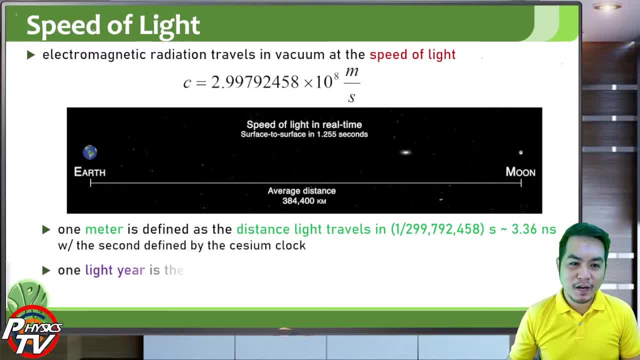 with the 1 second defined by the session clock. So one light year. there are so many misconceptions about this. One light year is not a time, it's not a year, it's a distance. So one light year is actually the distance that light travels. 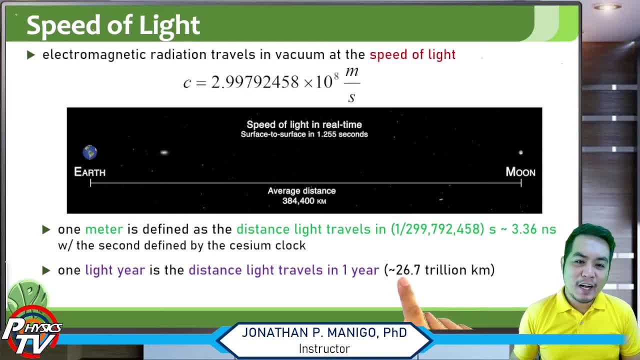 in one year, And that is approximately 26.7 trillion kilometers, So that's a very far distance. So, for example, the nearest star to us, Proxima Centauri, is around 4 to 5 light years away. So the speed of light. 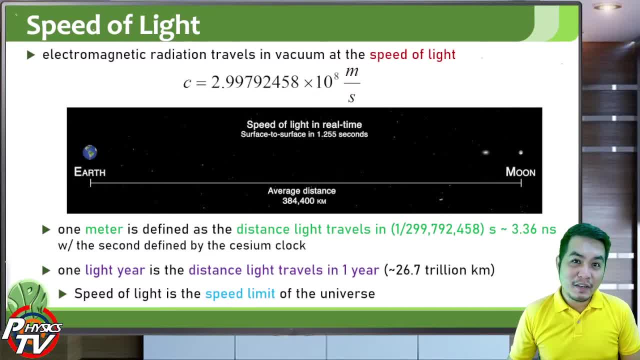 is what we call the speed limit of our universe. So nothing can travel faster than light as of now. No, but that is the theory states that that is the fastest, the fastest speed in the universe. It's the speed limit of our universe.